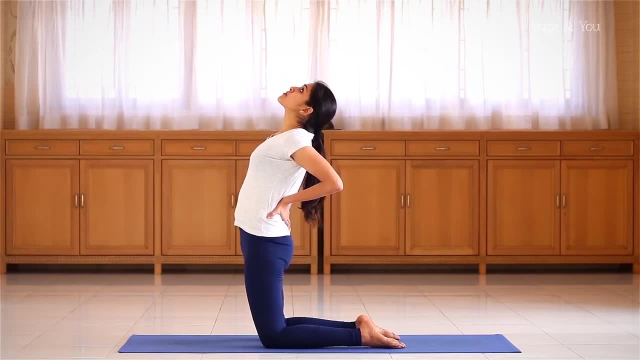 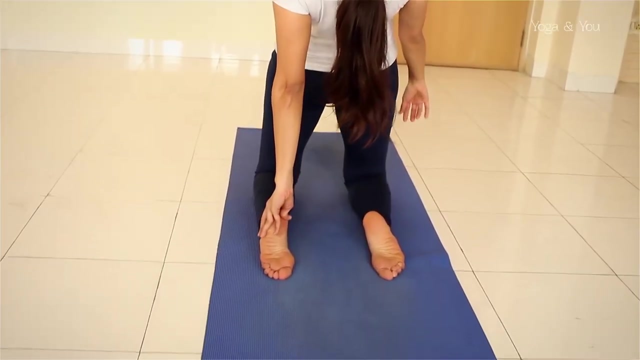 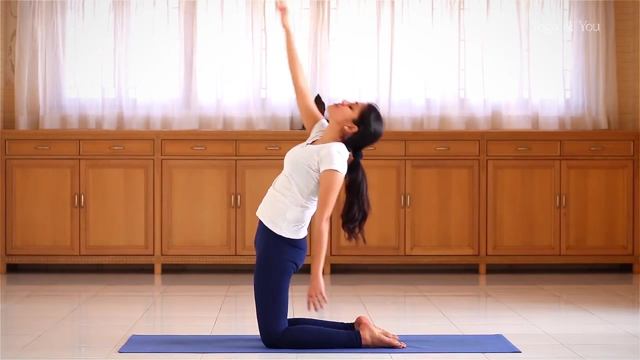 Place your hands on your lower back and arch back. This is the basic version of Ustrasana. Release. Now place one hand on the ankle behind, Take the other hand up towards the ceiling and look at the hand which is up. Release and repeat on the other side. 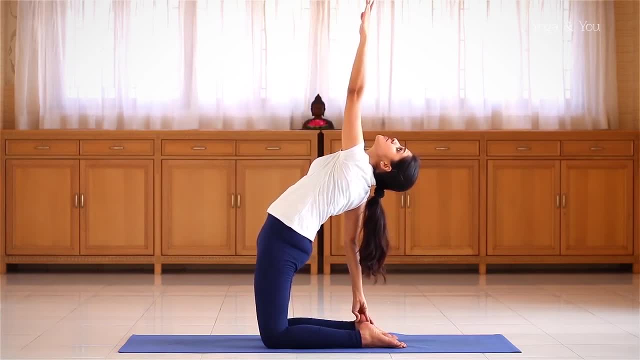 Ustrasana, Stand on your knees, with the knees slightly apart. Place your hands on your lower back and arch back Down, and move the hips slightly forward, up and down. For the complete version, place one hand on the ankle behind and the other hand on the other ankle. Push your hips forward and arch back. 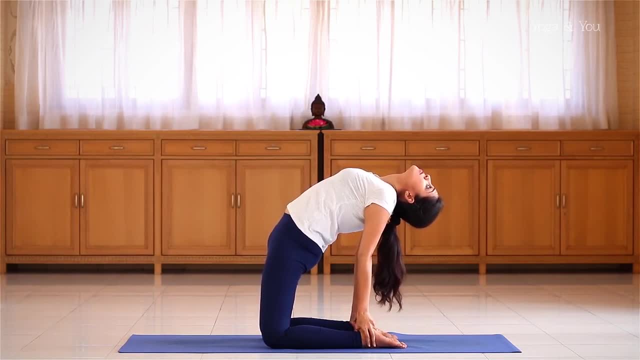 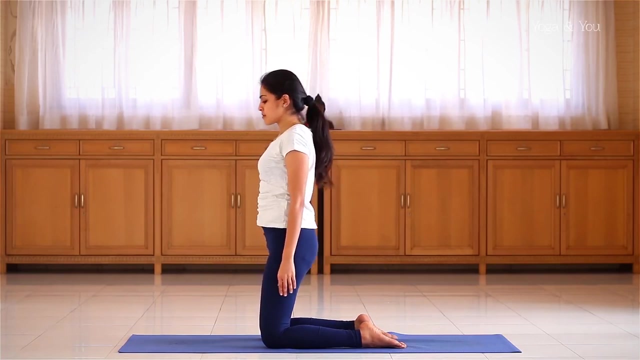 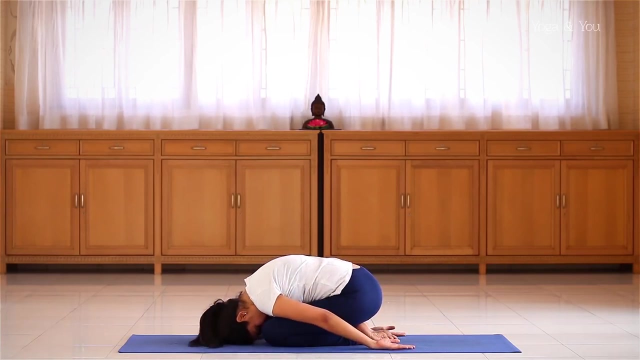 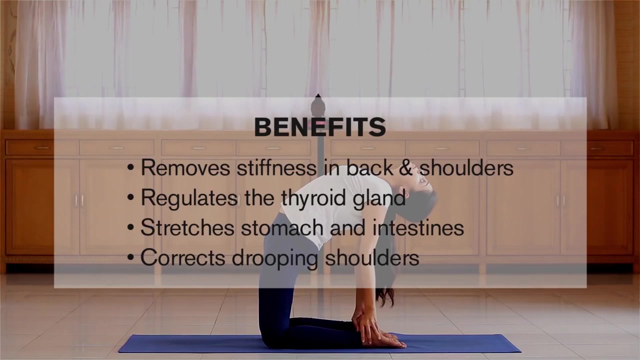 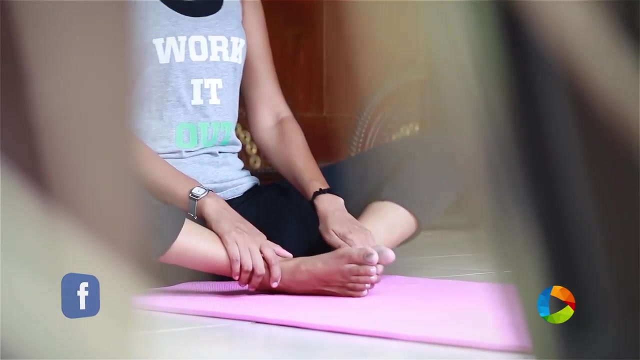 Look at the ceiling, Slowly release the asana And sit back and relax in child's pose. Begin to sit with a straight back and keep your soles of your feet together and interlock your fingers onto your toes and begin to flap your thighs. So 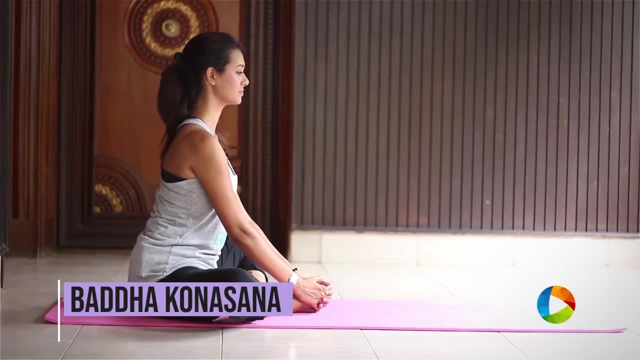 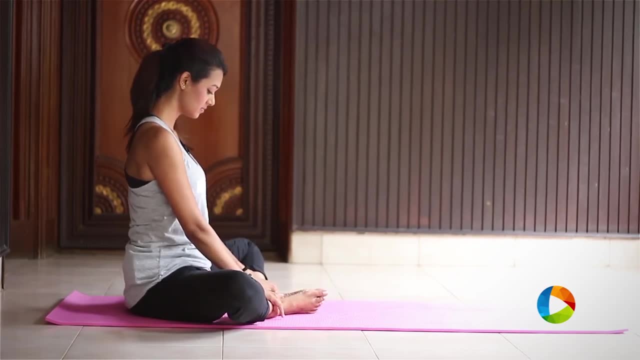 this helps in opening your tightness in your groins and your hips. Make sure your breath is really normal. To intensify the stretch in your groins, pull your feet closer to your pelvis and begin to flap for a couple of times. 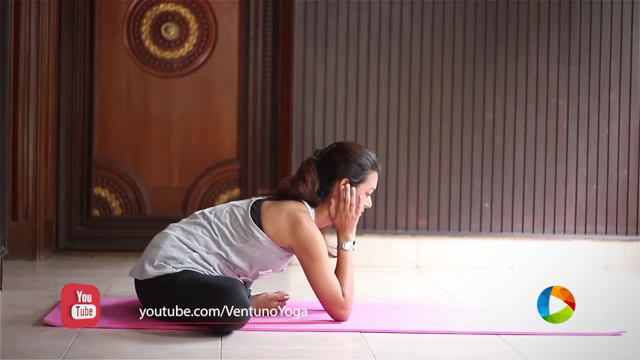 Now, if you are a beginner, slowly bring your elbows down to the mat and rest in this position and make sure to breathe. Now, if you are a beginner, slowly bring your elbows down to the mat and rest in this position and make sure to breathe. 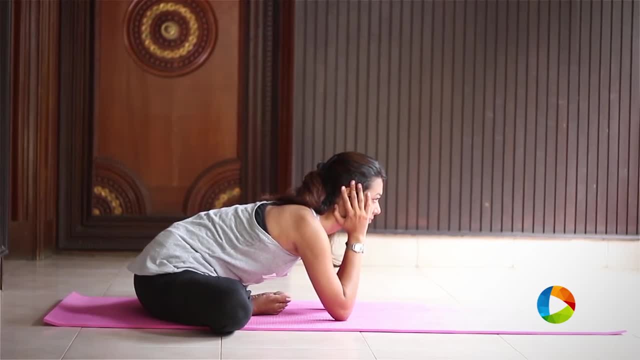 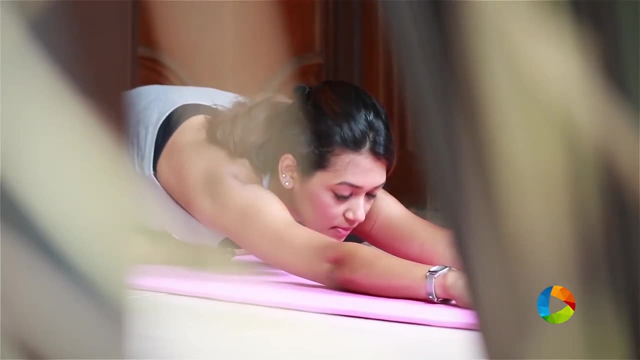 So that you are getting used to the stretch which is in your groin and your hips area. But to intensify the stretch even more, gently, stretch your arms all the way forward and put your forehead down to the mat. It is going to hurt the